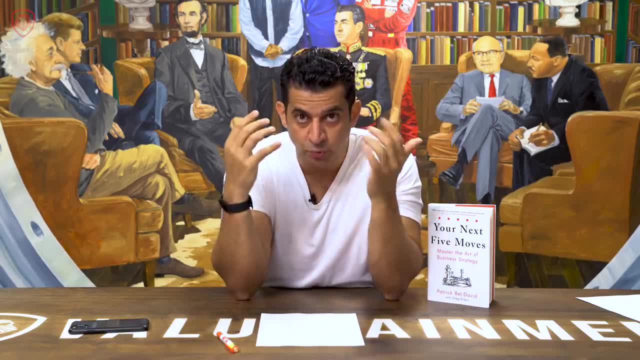 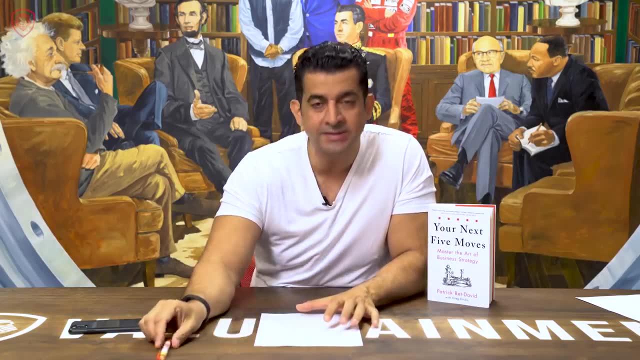 but what they lack is discipline, effort and a good attitude. This is why they keep becoming temps, And unless the effort, discipline and attitude changes, they're always going to be temps. The second kind are the ones that I call part of the 450.. 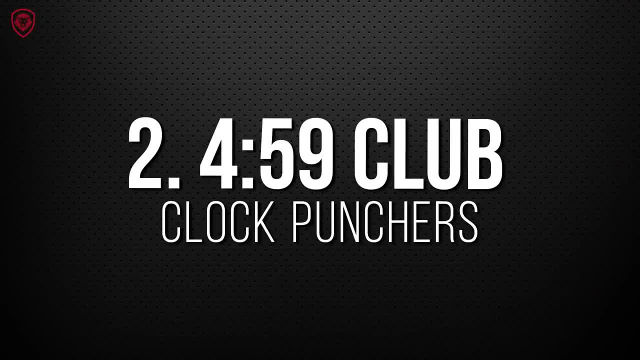 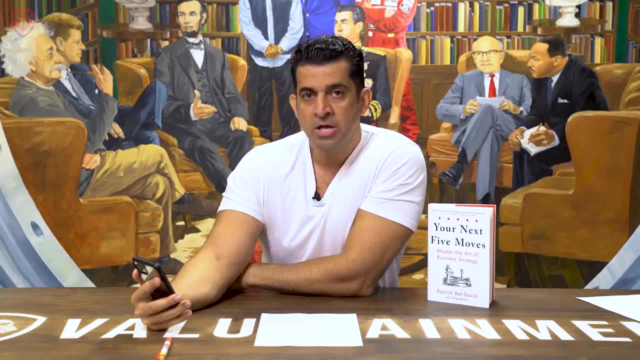 Club. Let me tell you what's the 459 Club. You know a lot of 459 Clubs. You may be part of the 459 Club. Here's who the 459 Club is. This is what they do. They look at the clock. They don't stop. 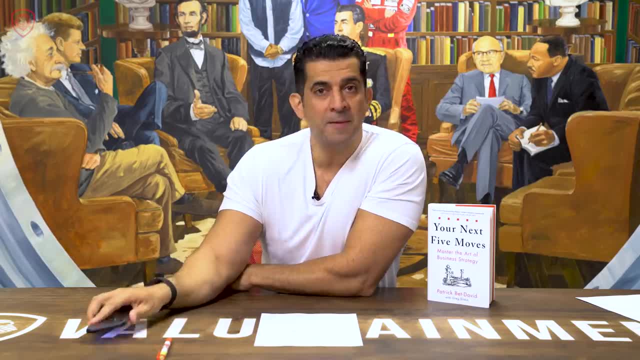 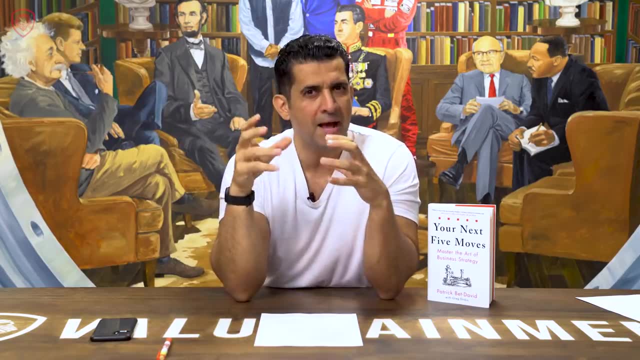 working at five, They clock out at 459.. Like by 445,, they already got a foot out the door. They can't wait to leave. 459, boom, they're out of here. So they'll do enough, whatever you ask them. 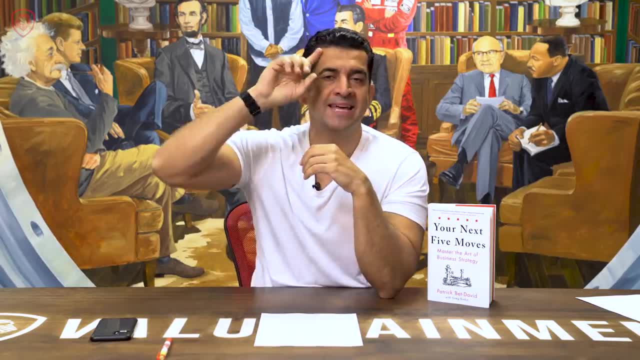 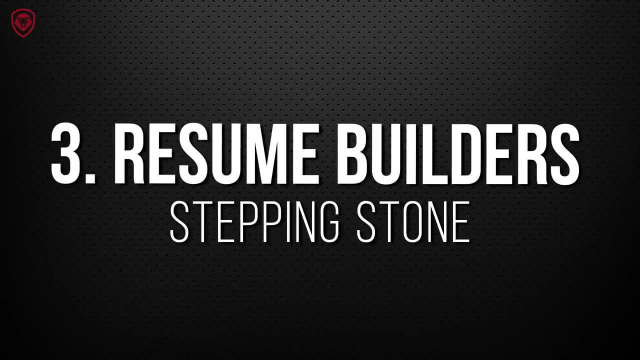 to do. They'll do some of their work. Most of the work they'll do it, but they cannot wait to leave this place and go do something else. The resume builder. Resume builder is somebody that goes works at a company for two years. gets some experience under their belt, then they go to the next company. They'll typically do this over a six to an eight year period to build up their resume, because they want to get that one job at a big four accounting firm or a big four financial firm. So they're simply building. their resumes. Nothing wrong with that. They still do their jobs, They're still good, but they're not going to be with you long term. They're just there to get the job done, build up their resume and they leave. And sometimes this actually works for both parties' favor, if you know. 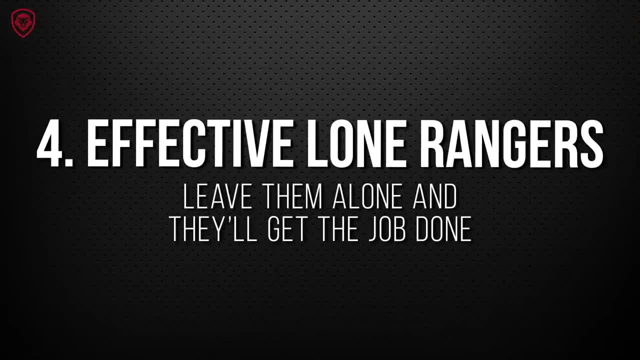 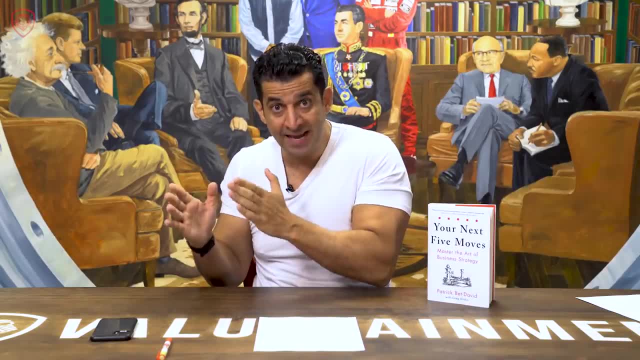 that this is what the expectation is. The fourth one is an effective lone ranger. What am I talking about with an effective lone ranger? This is somebody that doesn't want to be bothered. You give them the task, it's going to get done. They don't talk to a lot of people. They'll slip out. 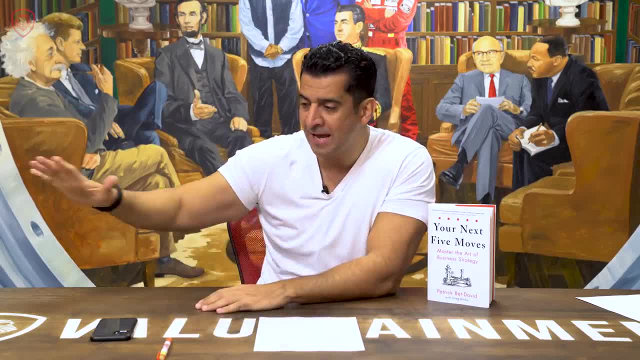 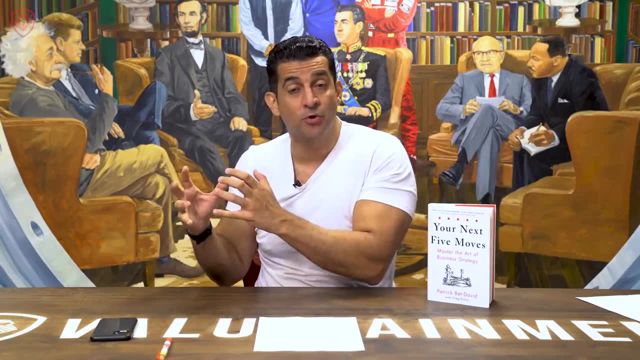 their cubicle or their office and they'll get everything done. It typically has to do with financing some creative work that's purely on the computer coding, a consultant that's coming in for a year and a half to just get the job done on a website that's being developed or a CRM that's. 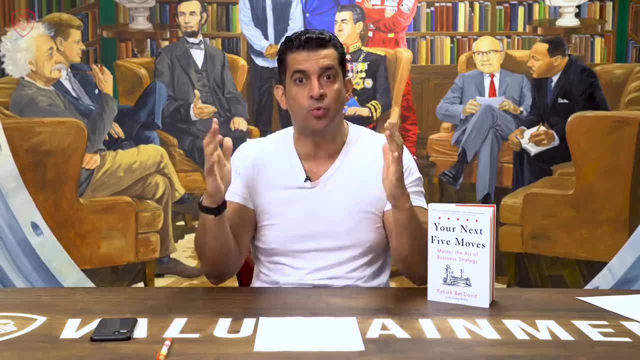 being developed, So they're going to get the job done. They're going to get the job done on a website that's being developed. Tell me what you want me to put together. Leave me alone, Let me get to work. That's the effective lone ranger. The fifth one are the team players. These are the guys that 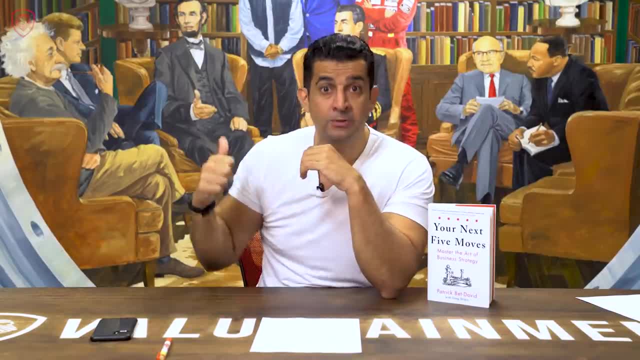 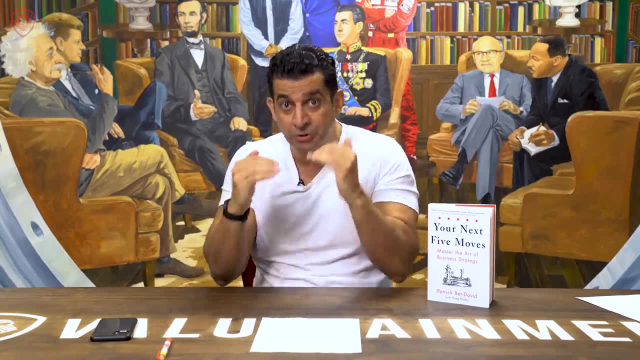 are willing to help out, no matter what happens. Look, what do you need? I'm willing to help out. Do you need me to come on the weekend and help out? I'm here. You need me to stick around a little later. I'm here. I got my job, then I can help out. Do you guys need anything else? These are. 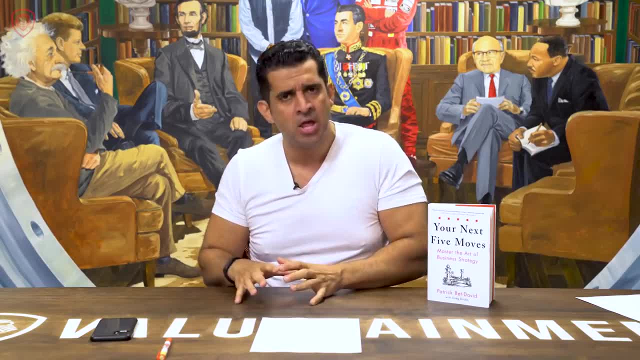 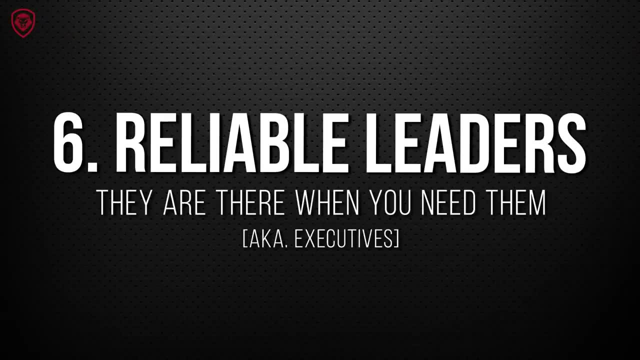 people that constantly get racist and eventually they could end up being a strong executive, but they're very good team players. Some of the most important people you can have at a company are team players. Number six are reliable leaders. What are reliable leaders? These are the executives and directors that will go and 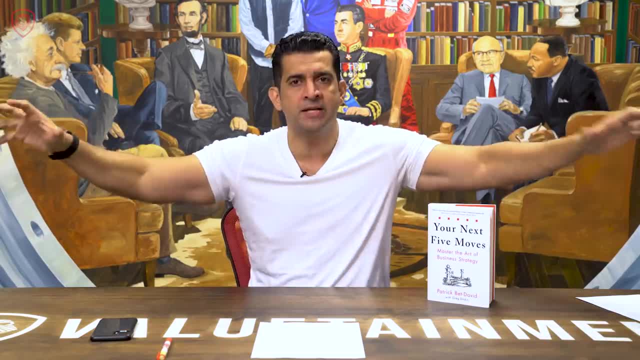 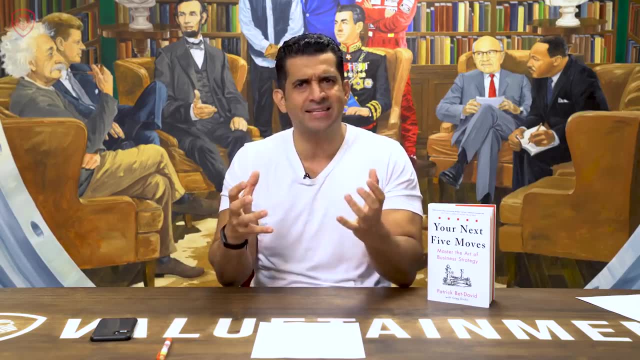 simply do the job you ask them to do and they'll manage their team. They will go above and beyond, They will do their part, They will lead well, They will manage well, They'll get the tasks done, They represent the company well And they could be with you for three, five, 10,, 15,, 20 years. 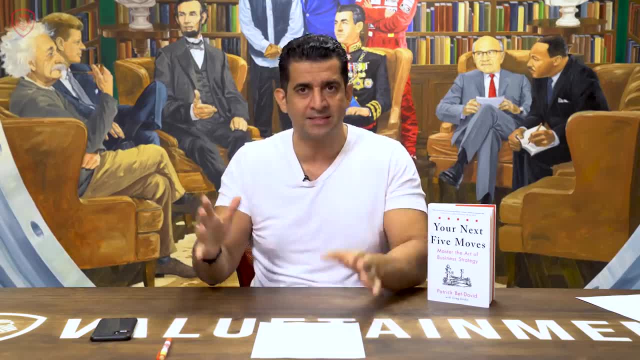 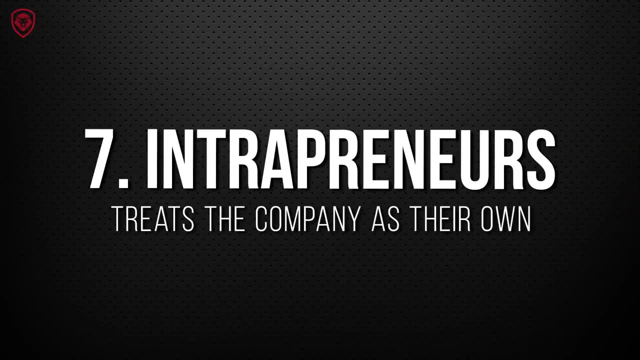 and be reliable leaders And they can be a very big asset to the company. And then you have the highest level of leaders At every company And these are the entrepreneurs. See, the whole concept about entrepreneurs is something I talk about in this book in chapter three. Everyone wants to be an entrepreneur. 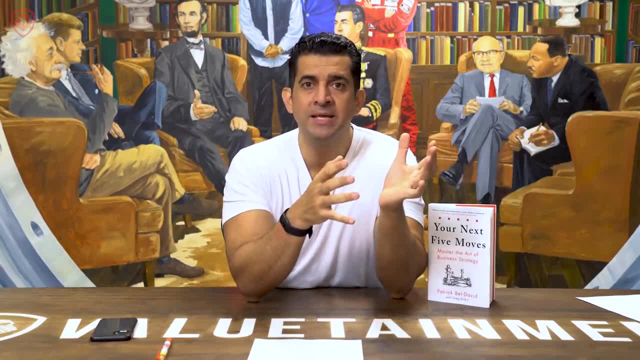 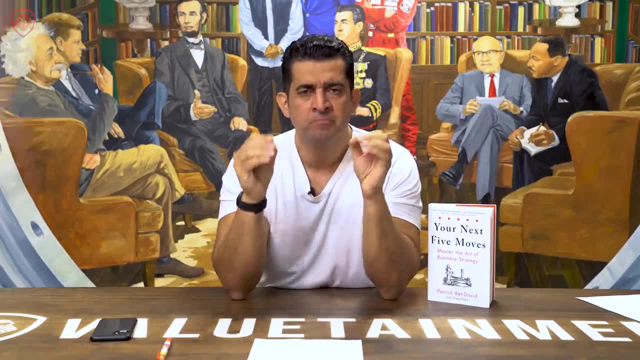 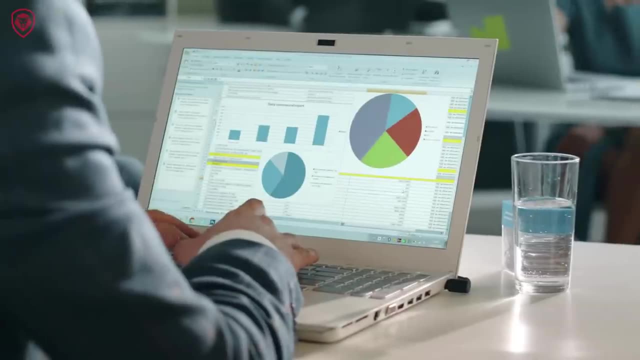 but sometimes you can have it all without risking it all, And that's being an entrepreneur. An entrepreneur thinks, walks, talks, everything they do. They think like the entrepreneur founder. They think like the person that started the company. The money to the company matters to. 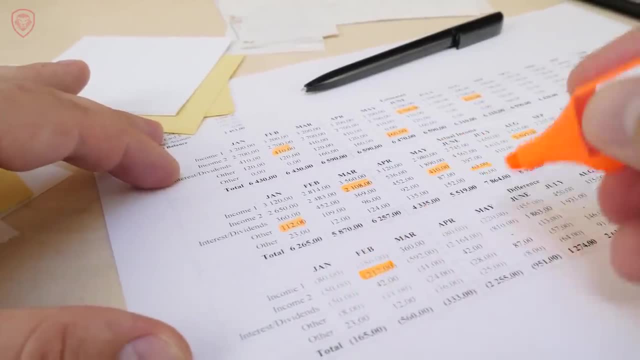 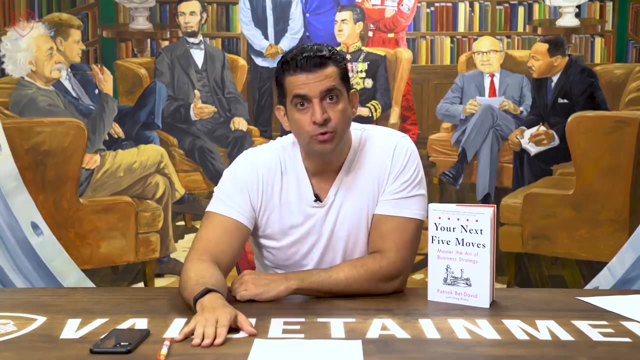 them. If you spend $1,000 here, they'll go on three additional websites to spend $850 on it. If we're going to spend $29,000 on a travel, they'll go shop it out and bring it down to $2,600, $200. 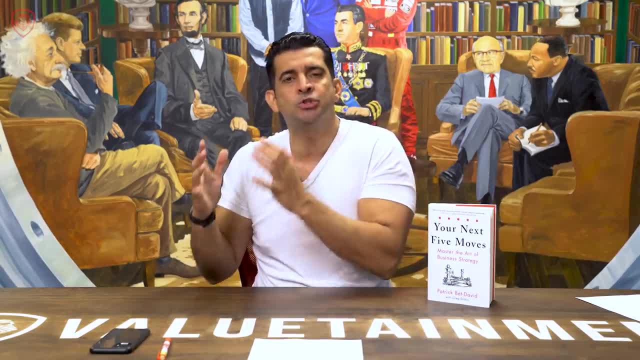 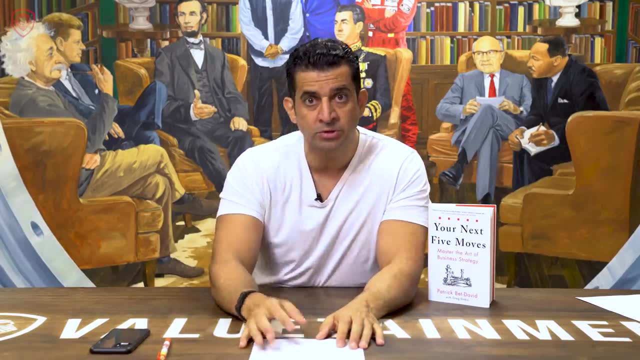 just to save $2,800.. It doesn't matter what it is An entrepreneur. everything they do with the company, they treat it like their own. You know what typically ends up happening to entrepreneurs: They end up becoming C-suite executives, They end up owning equity in the company and end up 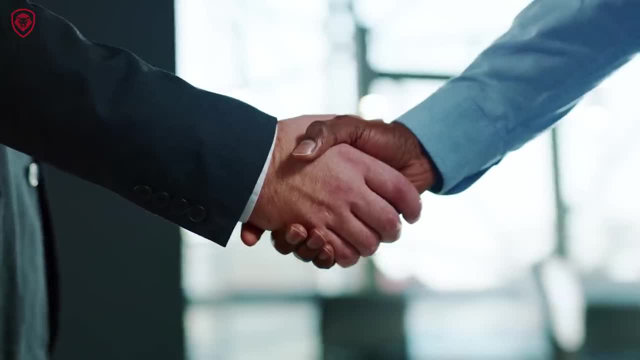 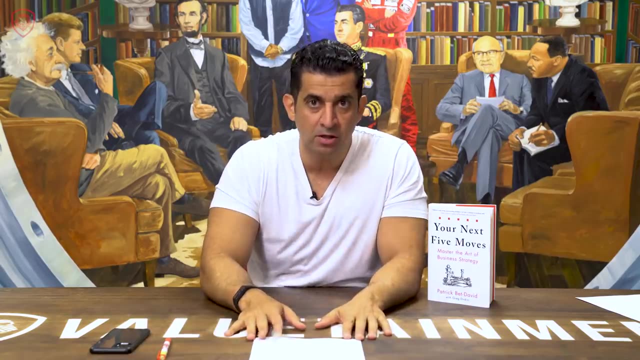 eventually, many of them running the company, if not running a part of the company, running the division of the company because of the way they're wired. So these are seven different types of employees and team members at every single company. A couple things I want you to do. One: 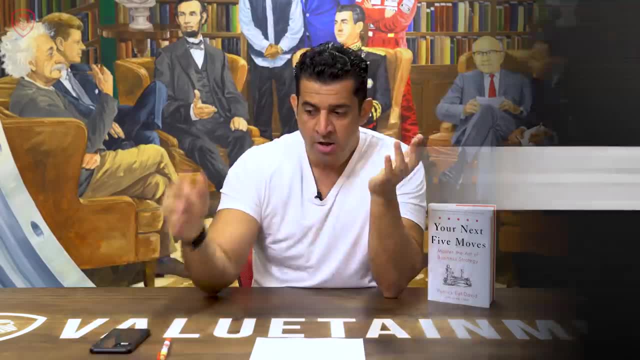 I want you to ask yourself which one you are. And, by the way, no one's watching you, No one knows where you are. You may be at work listening to this saying: I think he's talking about me. I'm a level two. I think he's talking about me. I'm a temp. I'm always getting fired. Maybe it's not. 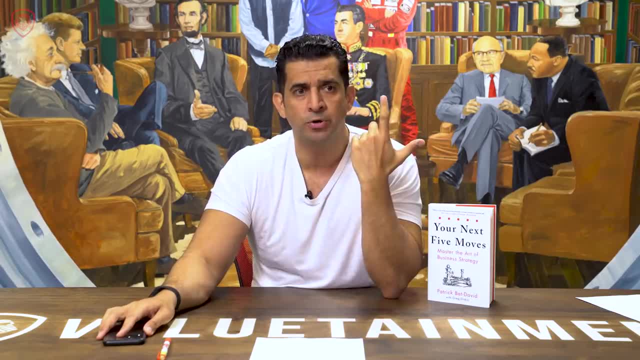 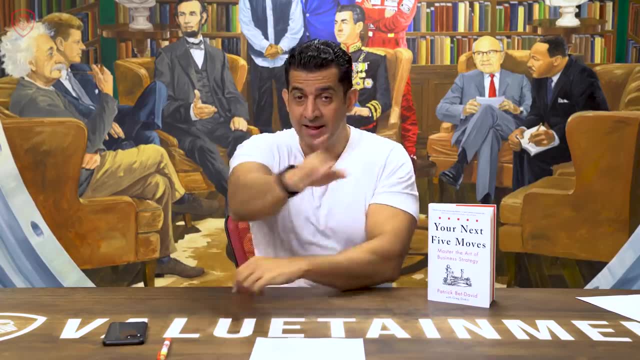 the company's fault. I think I'm a level four. I don't think I'm an entrepreneur yet. I think I'm reliable. I just don't think I treat the company's money like my own. Maybe I got to upgrade Whatever it is, think about it. 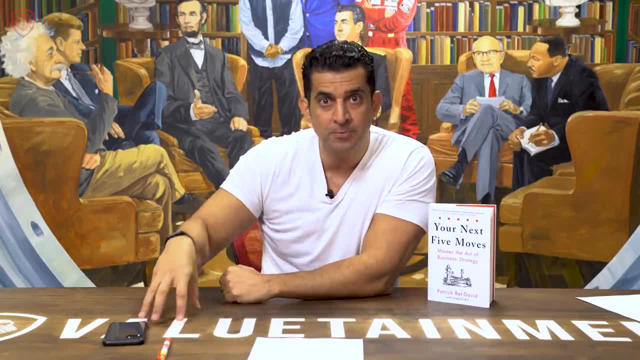 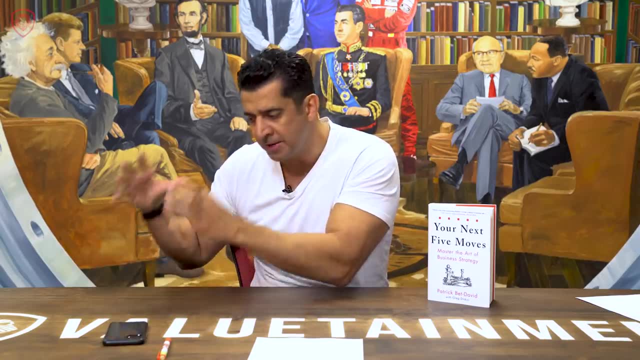 And then, if you're a boss and a CEO and a founder, think about all the people you have in your company, who falls in which category and who needs more time with you, because those are the ones that could be the future of the company. That's where you need to invest your time and your capital into.